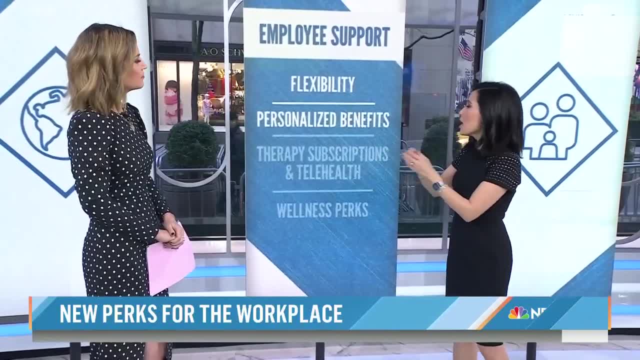 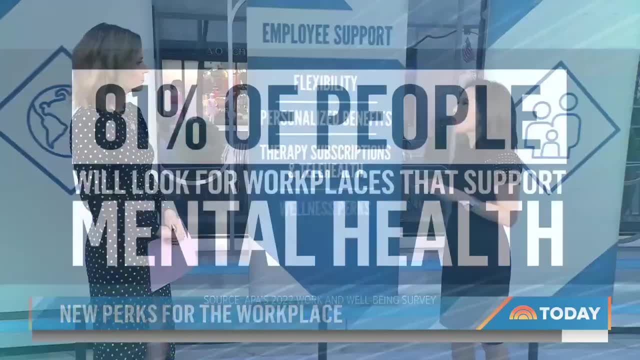 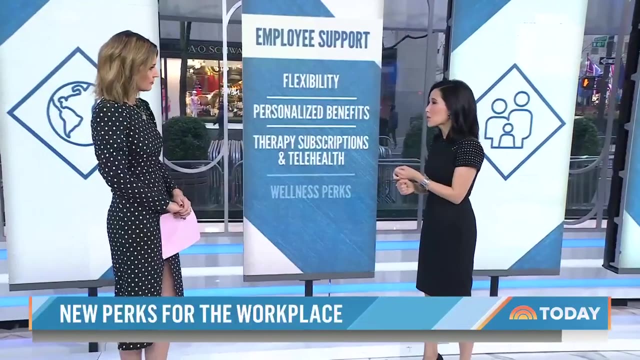 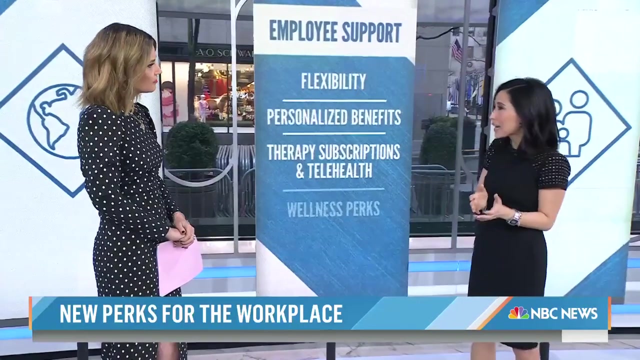 tennis lessons. Why not apply that stipend to you as well? The other thing we're seeing is the American Psychological Association did a survey and eight in 10 respondents said mental health benefits are very important to me when it comes to my employment. So you're seeing employers say, okay, we're going to lean into that, We're going to pay for your talk space subscription, which is a talk therapy subscription, or your headspace, which helps you meditate instead of Medicaid, And you're also going to see the continuance of telehealth, which became really popular over the pandemic. That's sticking. 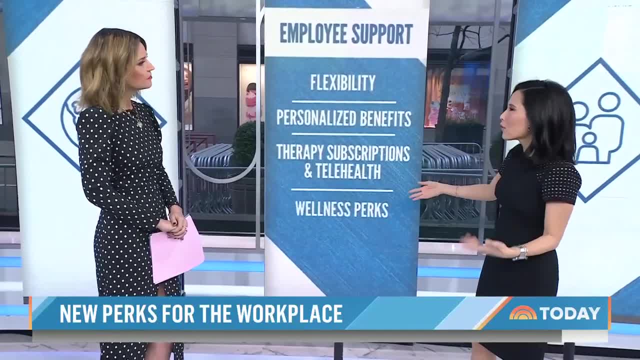 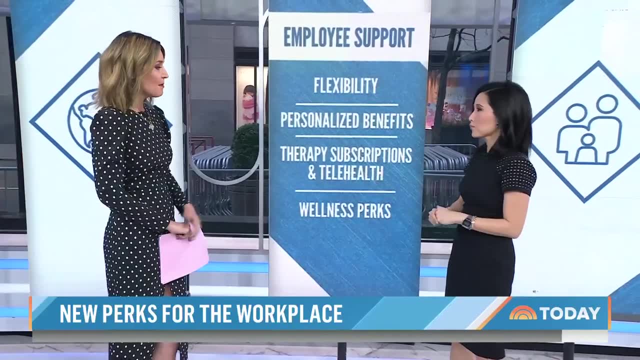 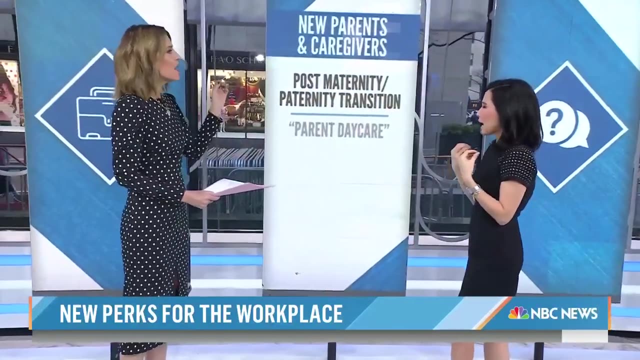 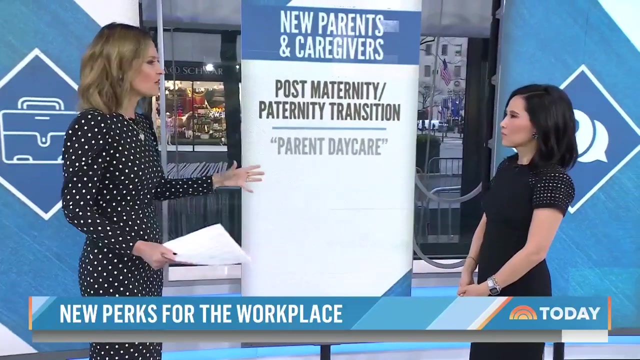 around And finally, things like meeting free Fridays or even a bonus for you to take your time off, your full time off for the year, instead of just working through it, as some people do. Yeah, I mean it makes sense for the employers too, because they're investing in you and hopefully it will be, you know, a good investment for the long term. Absolutely Happy workers means more productive. Now, you said a minute ago, or I said, parents daycare. I mean, we know about parental leave, but this is this category- is expanding this family. It really is So, as we are seeing paternity and maternity leave match up and 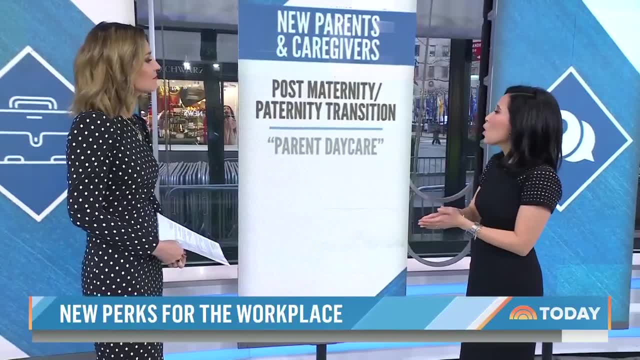 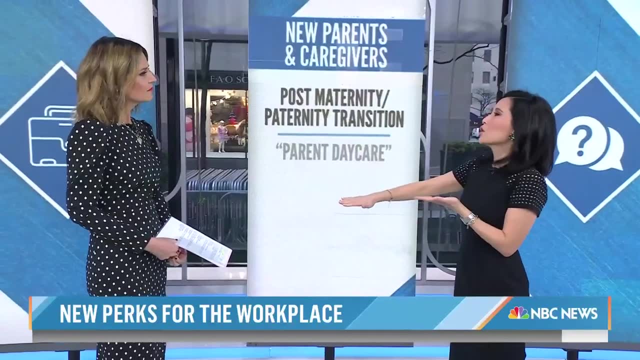 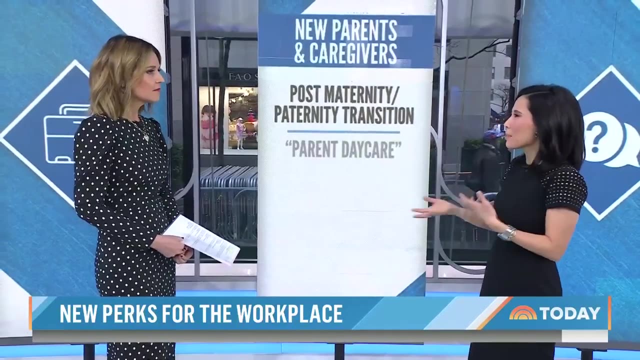 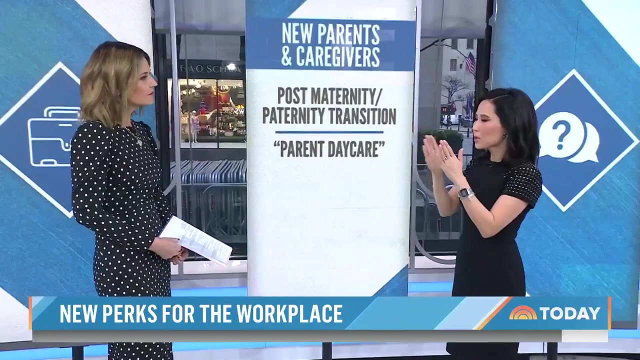 also time off for people who adopt or have a baby via surrogate. We're also seeing this thing called post maternity paternity transition, where they're allowing you to sort of ease back into your, your job- maybe not come back full time- two, three days a week, which actually makes that reentry a little bit better. I mean, you know, coming back to work, it's kind of nice to have a little bit of flexibility. Parent daycare is a huge one, So AARP did a survey and found that between the ages of 40 and 49, the workforce- more than half of us- are taking care of an aging parent. So the 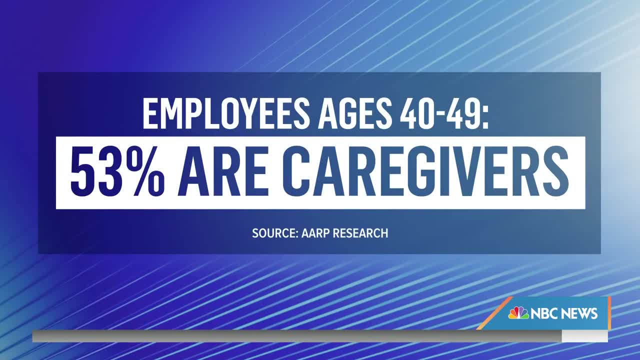 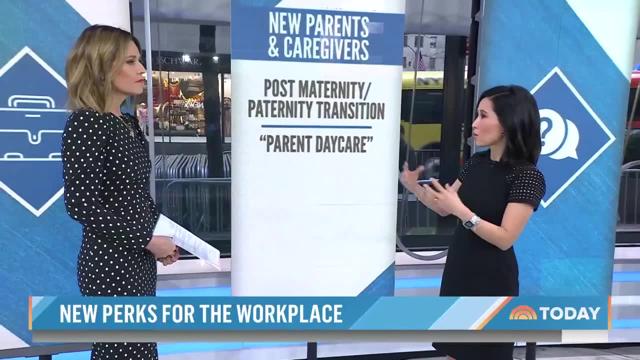 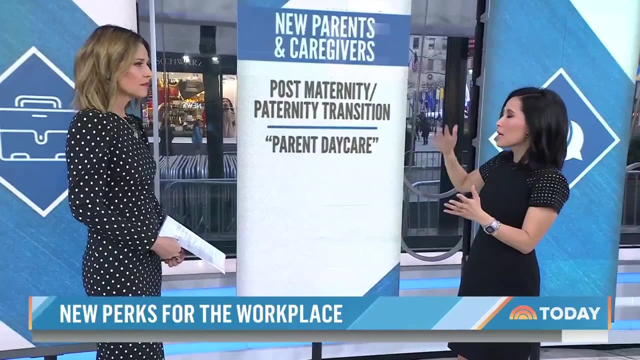 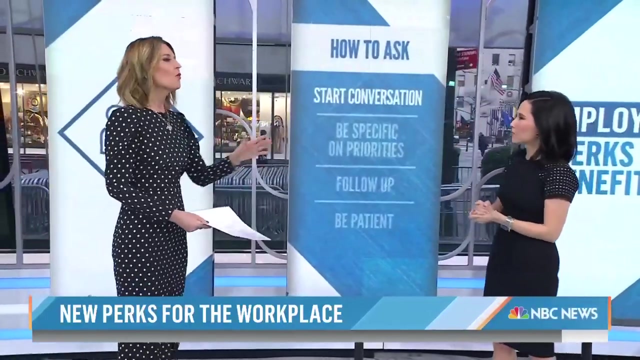 idea that you might be able to take your parent to a subsidized care center that the employer is shipping into So you have peace of mind at work, improves their life, your life and overall the company's culture. So that's something to look for. parent daycare- We've seen it with little kids, but now we're seeing the sandwich generation needing to care for elderly parents as well Makes a lot of sense because people have to miss work to take care of aging parents. So it does make sense. What if you don't think you have any of these things, You don't think your employees offering it? How do you ask or start that conversation?